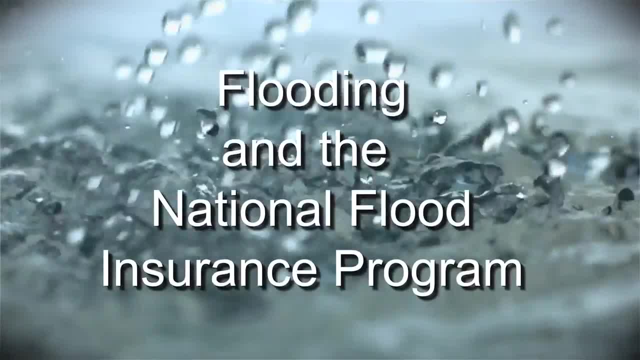 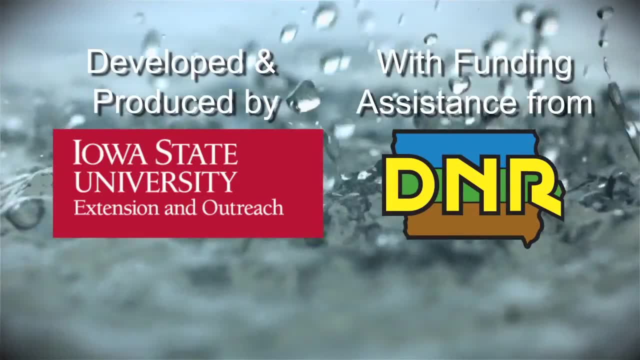 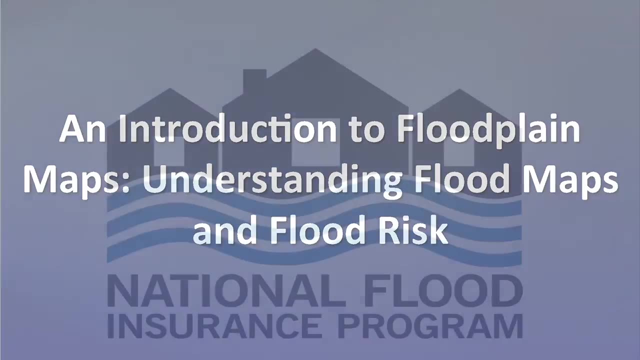 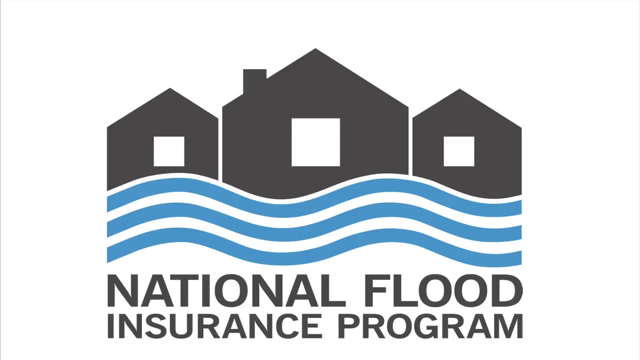 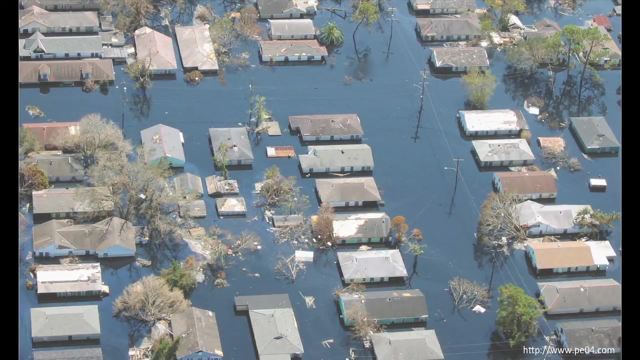 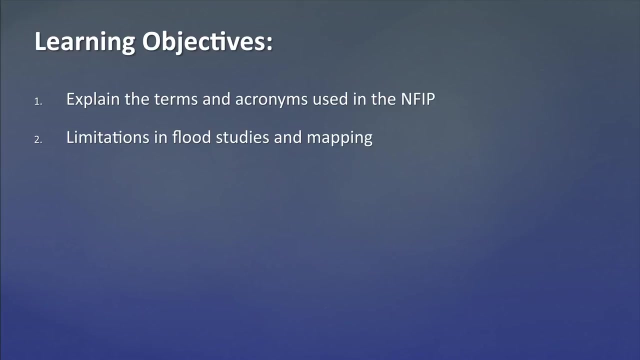 As you know from viewing other videos in this series, there are many terms and acronyms used in the administration of the National Flood Insurance Program, or NFIP. Many of these terms are meant to express notions of flood risk. In this video, we will explain the terms and acronyms used in the NFIP that are most critical. 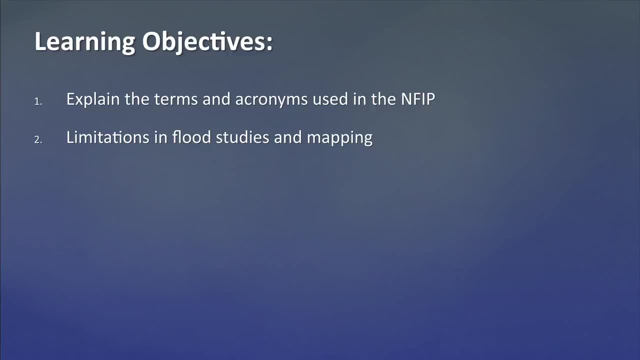 for understanding concepts of flood risk and explain the limitations in the ability of flood studies and mapping to express the real risks faced by property owners. These key terms and acronyms will be used during this presentation. You can find the terms and their definitions at the web address on screen. 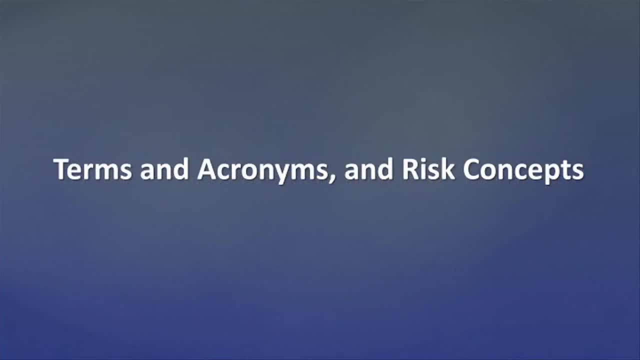 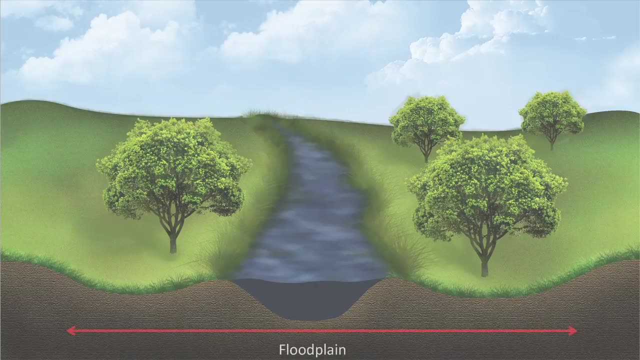 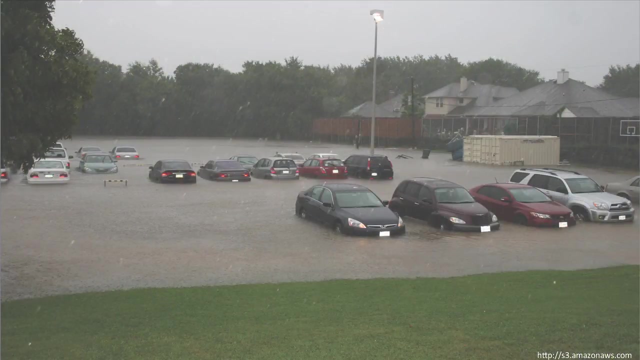 Rivers, streams and lakes are expected to flood. As a result, all bodies of water have floodplains, As we discussed in Video 7,. however, many factors affect the depth, duration and frequency of flooding for any given water body. 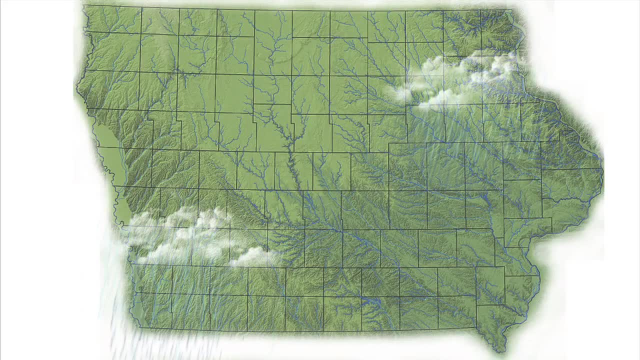 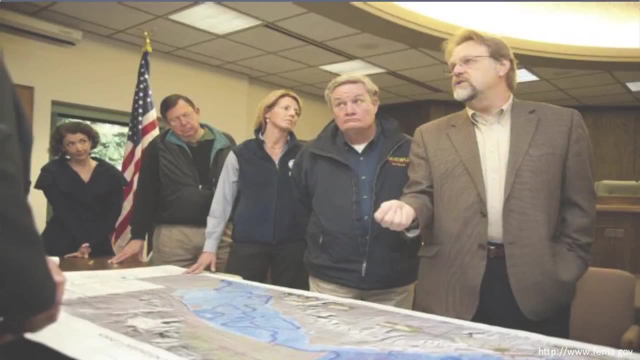 Because of this, the same amount of rain falling over the same period of time in two different watersheds is likely to result in very different flood events. FEMA's Federal Insurance and Mitigation Administration is charged with identifying flood-prone areas in the United States and establishing ways to quantify the actual risk of flooding within. 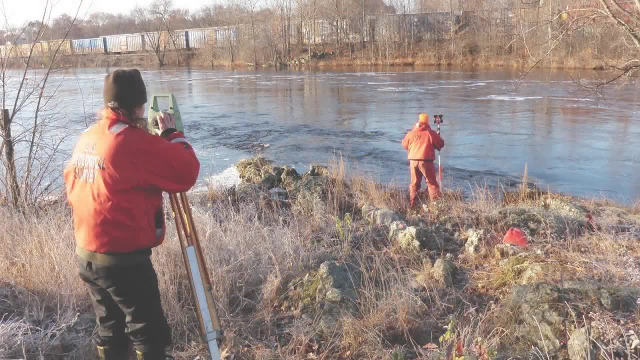 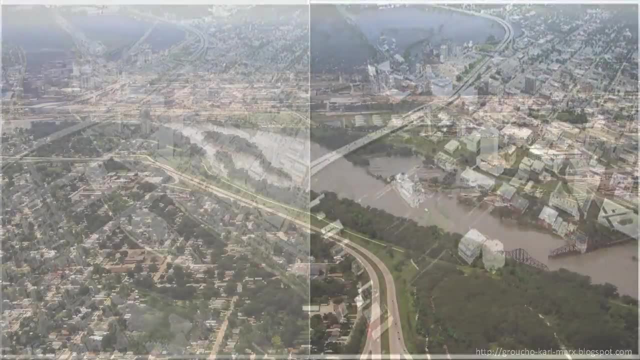 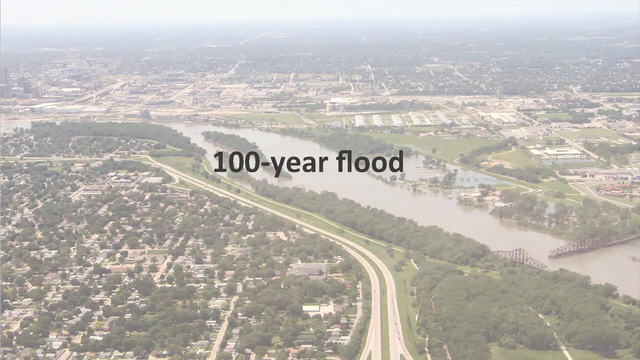 those flood-prone areas. Studies are conducted to estimate the inundation areas for both relatively common and less frequent flood events for the same water body. The most commonly referenced representation of risk in the NFIP is the concept of the 100-year flood. 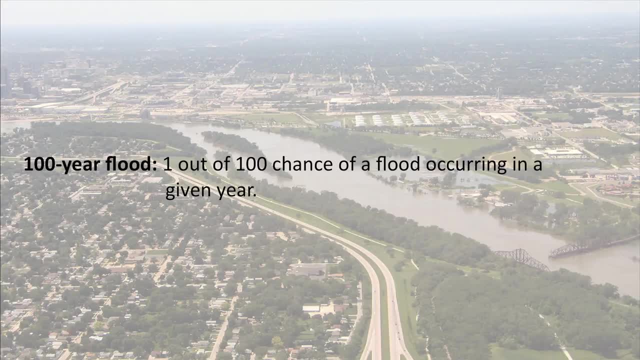 The 100-year flood is the flood that, based on statistical probabilities, has a 1 out of 100 chance of occurring or being exceeded in any given year. Unfortunately, the term 100-year flood is too often interpreted to be a prediction that. 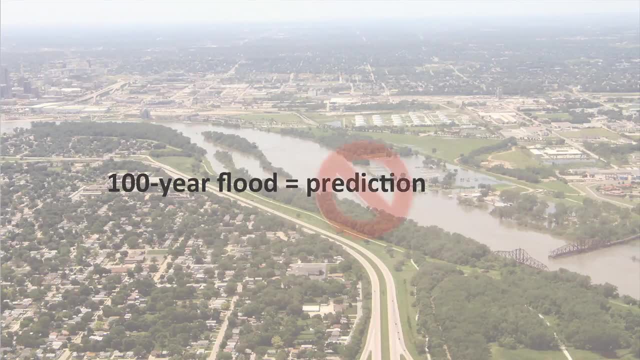 such a flood could only happen once every 100 years. when, in fact, when it is meant to express the probability of the flood occurring, The 100-year flood is also referred to as the 1% chance flood, which is a more appropriate 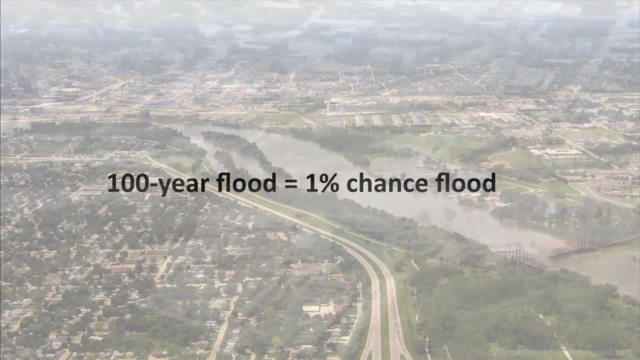 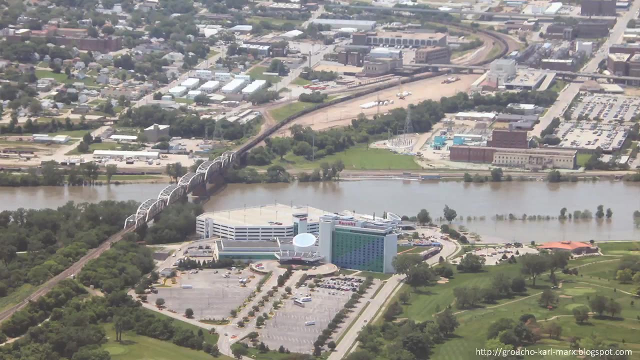 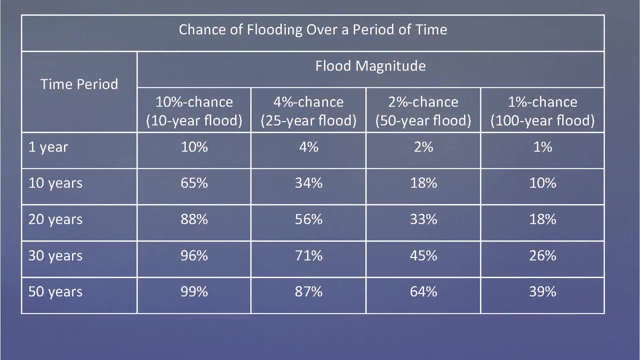 description of the risk of such a flood occurring in any given year. A river could experience a 100-year flood, twice in the same year, three times in 10 years or only once over the course of 250 years. The table on screen helps explain the concepts of flood probability and risk. 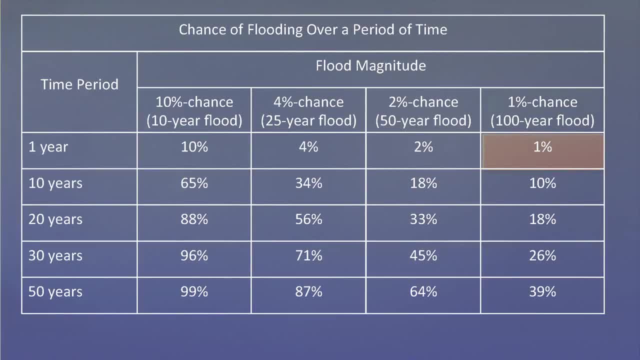 For example, the table shows that while there is a 1% chance of a 100-year flood occurring in any given year, there is an 18% chance that such a flood will occur within any given 20-year period and a 26% chance that such a flood will occur during the life of a 30-year. 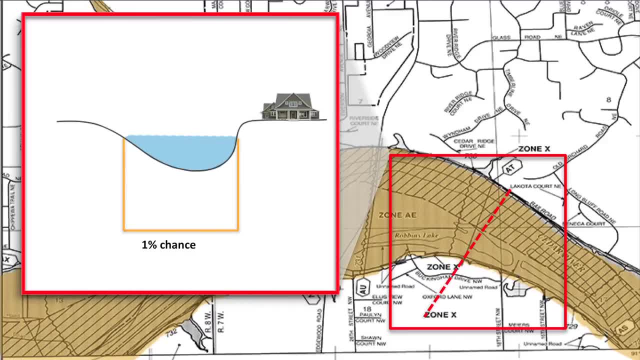 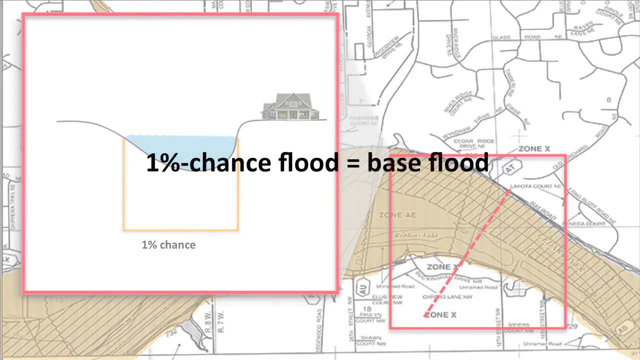 mortgage. In order to develop a common standard for the entire country, the NFIP adopted the 1% chance flood as the base flood for both insurance rating and regulation. The choice of the 1% chance flood was a compromise between using a smaller flood event say a. 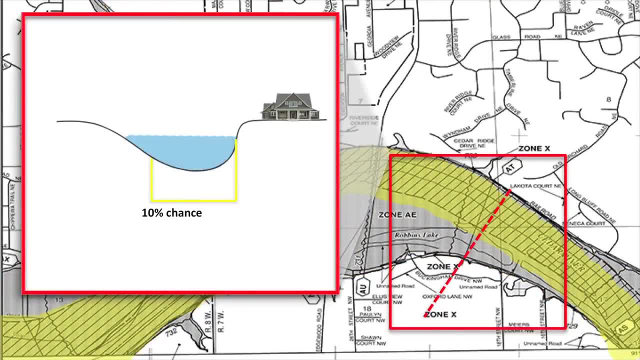 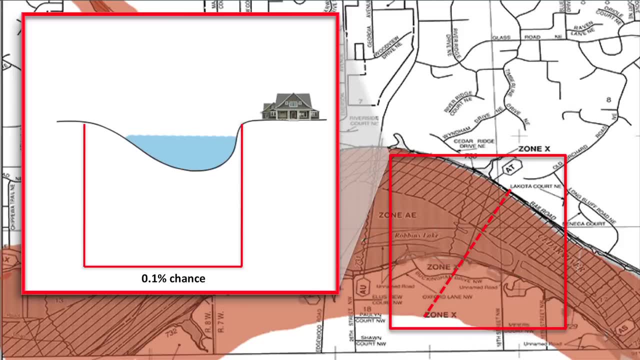 10% chance flood, which would leave many properties exposed to more frequent damage by flood and a larger, less frequent flood event, such as a 0.1% or 1,000-year flood, which was considered to be too stringent and an unreasonable requirement for most types of development. 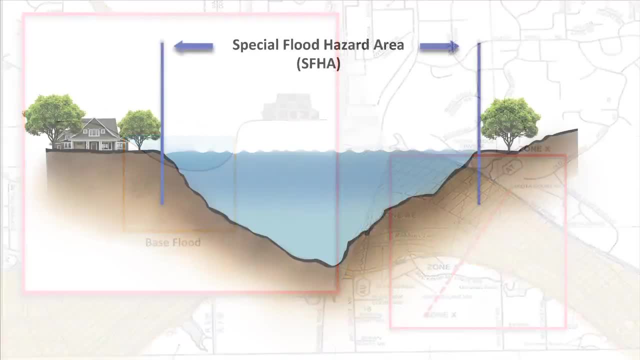 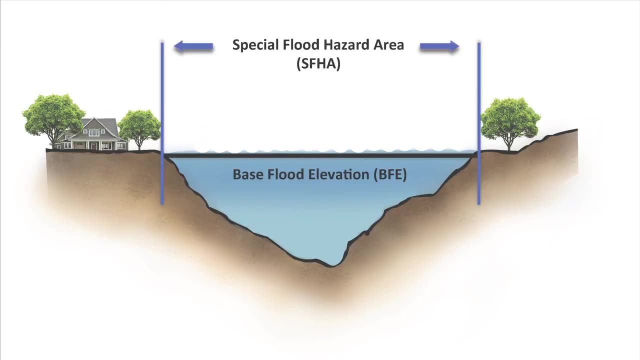 FEMA refers to the area inundated by the base flood as the special flood. The NFIP defines the base flood elevation, or BFE, as the elevation that floodwaters would reach at a particular location during the base flood. The methods for determining the base flood, the special flood hazard area and the flood. 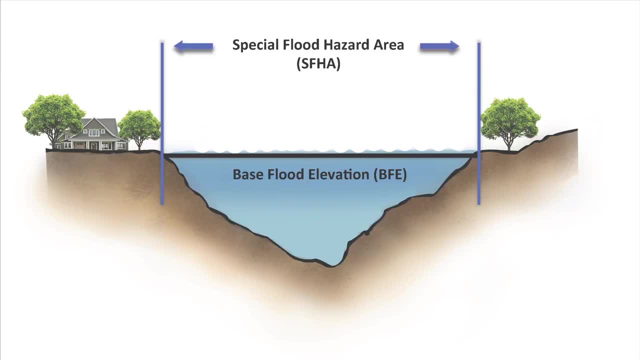 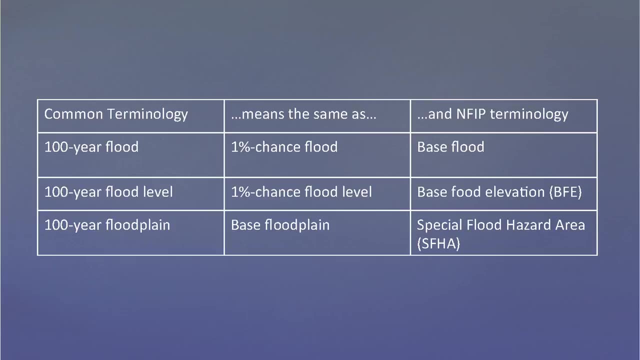 mapping process in general will be discussed in greater detail in Video 9 in this series. The table on screen shows the relationship between the two The terms used by the NFIP to describe the same concepts. From this point forward, the term base flood will be used to reference the concept of the. 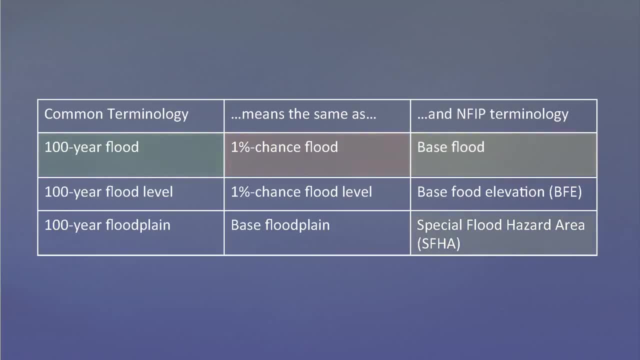 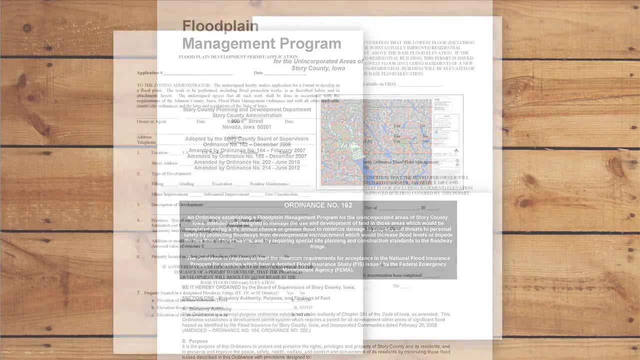